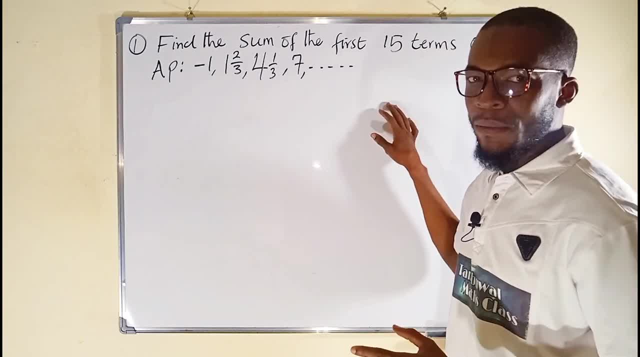 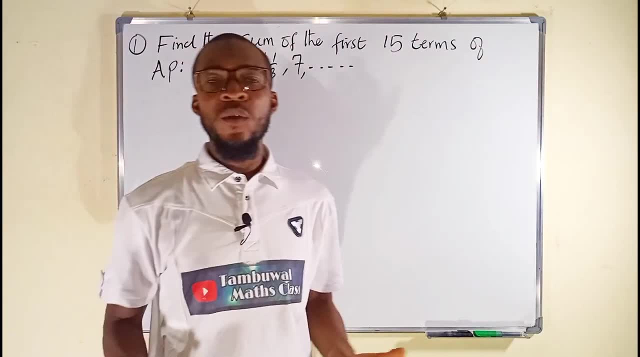 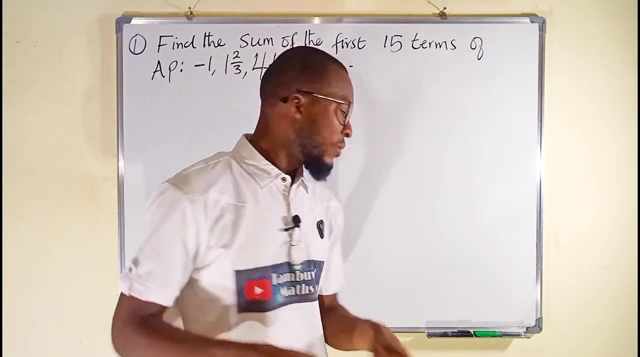 the number of times here, because there are infinitely many, but we only need the first 15 times. Remember, I gave you two formulas. or let me say we drive two formulas and to find out the right formula to use, it depends on the data given to us. So let us write our data first. 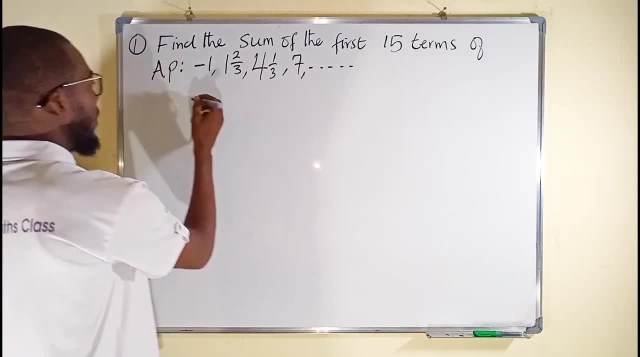 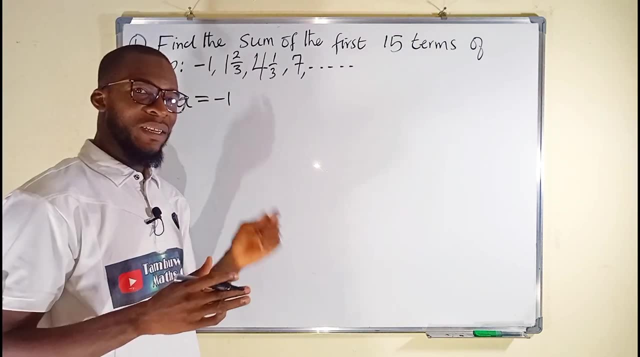 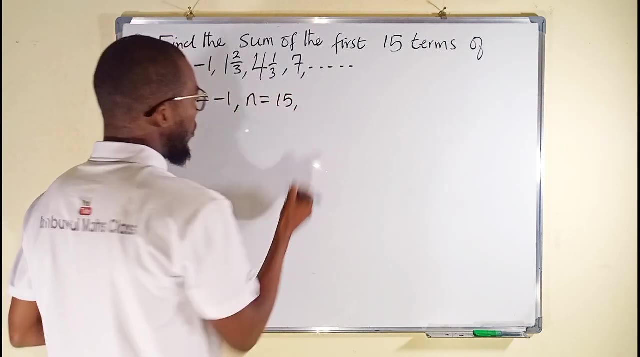 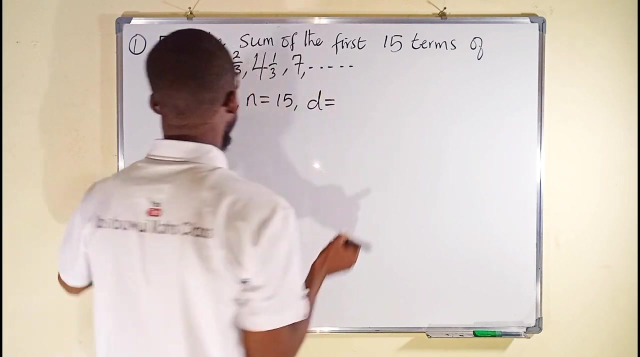 From this sequence you can see the first term which is donated by A is equal to negative one. Remember, we are interested in the first 15 times. Therefore our n is equal to 15.. Other thing we need here is common difference d, and how can we get that? We can take any of 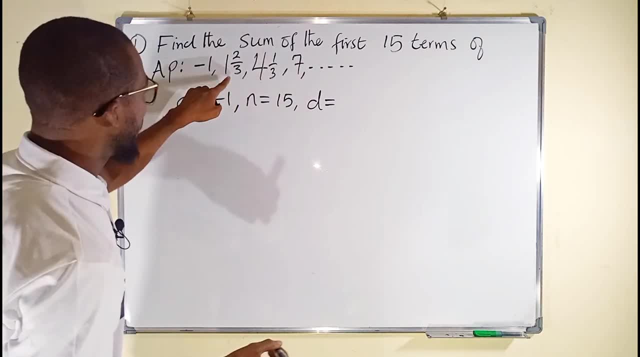 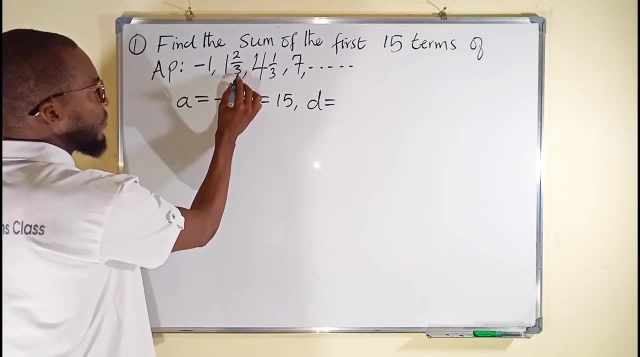 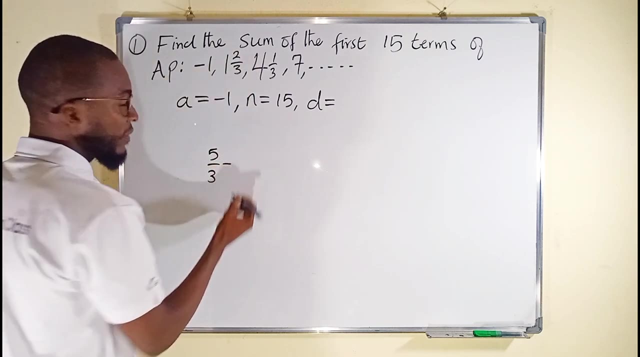 these terms and subtract the previous term. Let us take this one, which is one two over three. Let us convert it first of all to improper fraction: Three multiplied by one is equal to three plus two is five. So we have five divided by three, minus the previous term which we have. 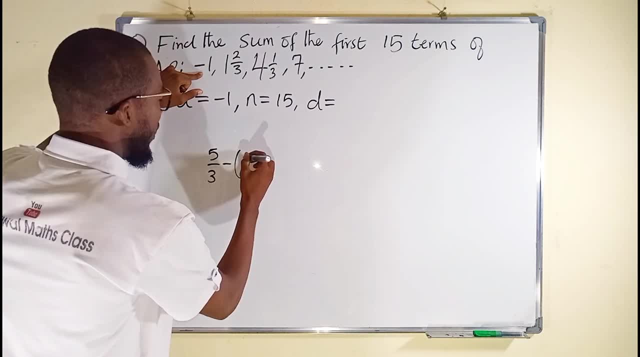 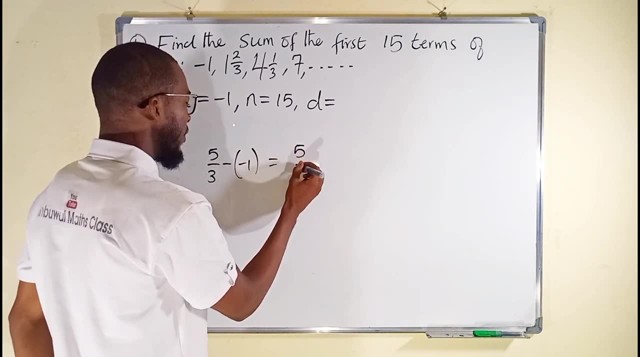 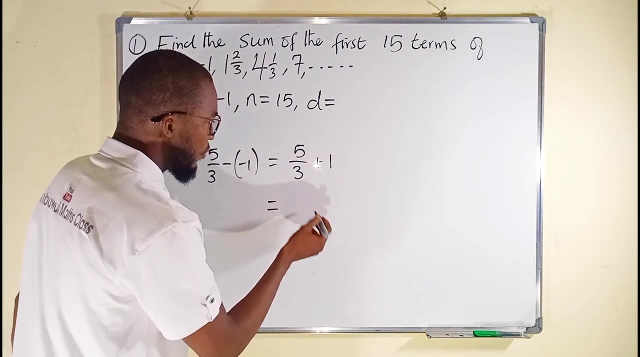 here as negative one, So negative one. this is equal to- because of this negative, negative, we have positive sign. five divided by three, m plus one. This is equal to eight over three. If you add this to this, you are going to get five divided by three. So this is equal to eight over three. 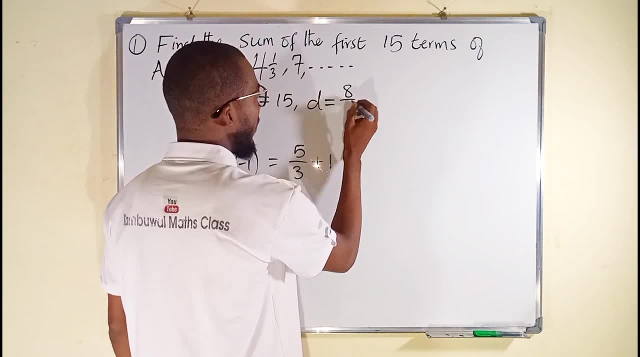 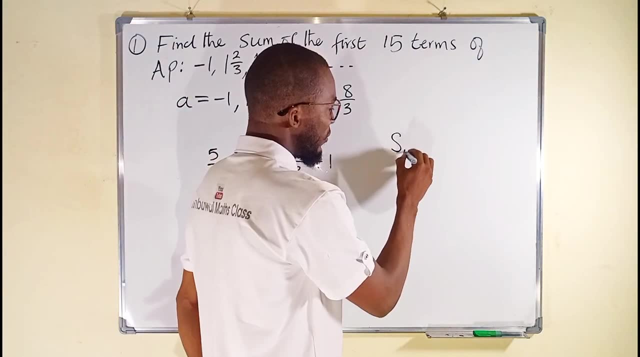 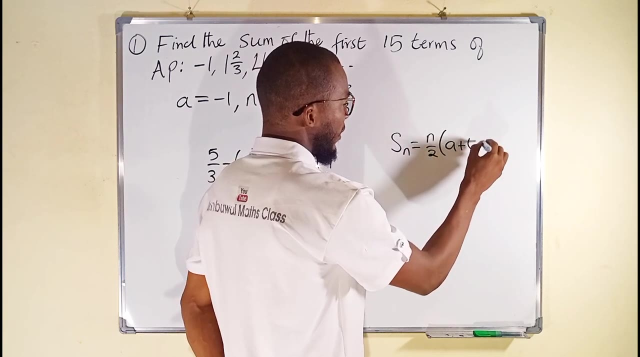 Therefore, our common difference is eight over three. So the two formulas. let me write all of them. The first one is sum of these terms equal to n divided by 2 a plus l. This is the first one. The second one is, as n. equal to n over two multiplied by two a. 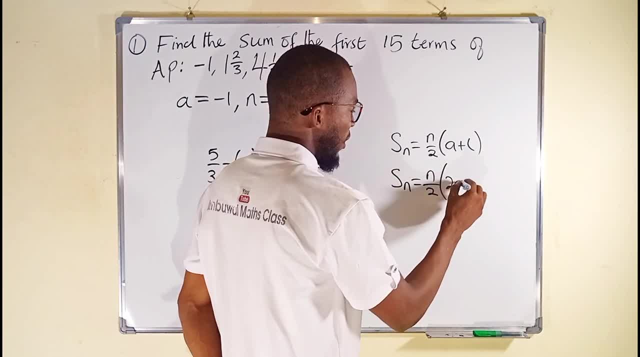 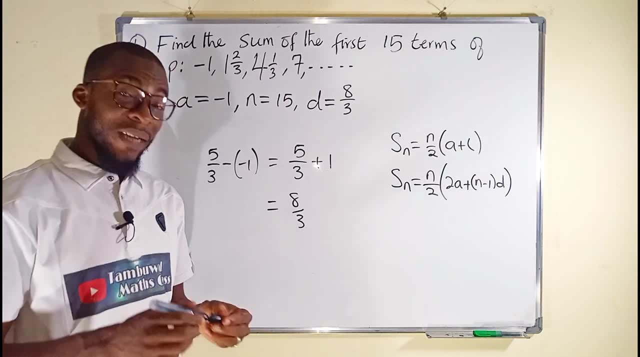 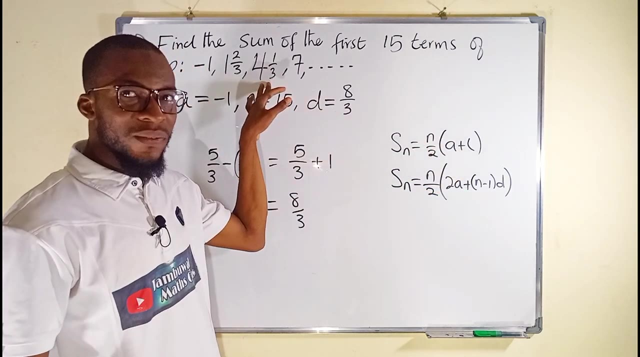 plus n plus l means 6 odd minus one multiplied by D. So it depends on the data given to you. You can see, in this first formula we have the last term, But the last term here is absent. Therefore we can't use this formula. 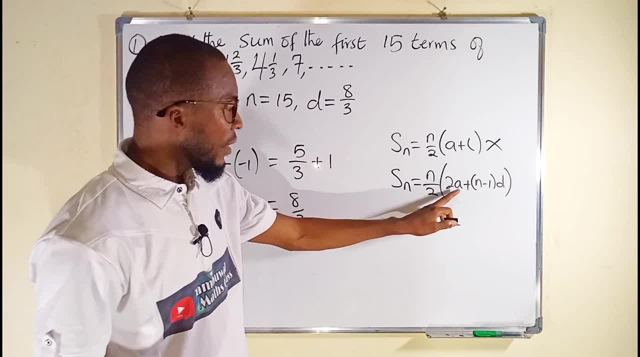 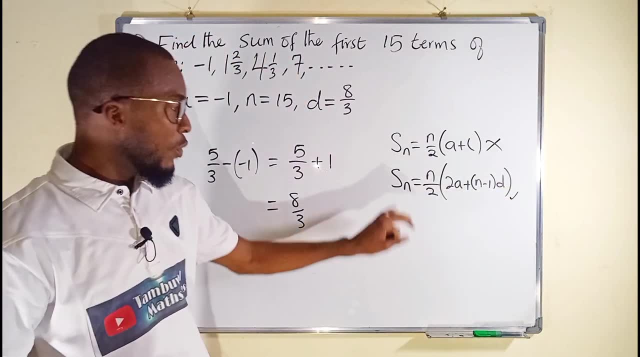 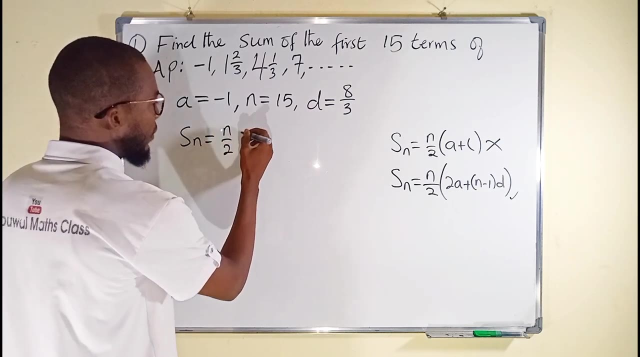 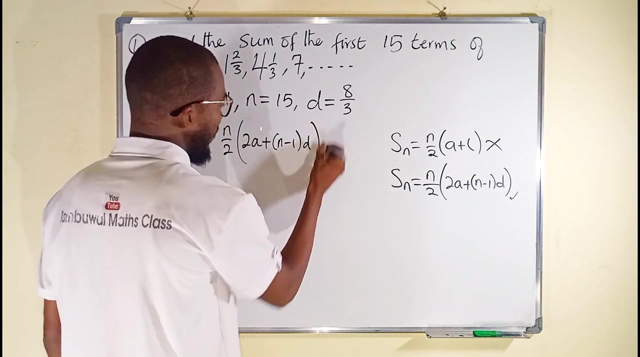 Here we are given N, which is this A? is this D? is that? So? everything we need is in this formula, So we are going to apply this. So S N equal to N divided by two, Two A plus N minus one times D. 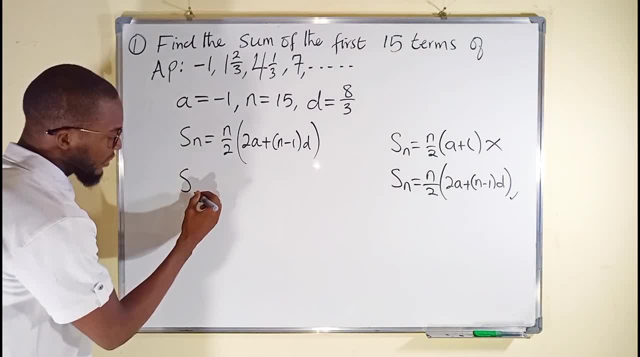 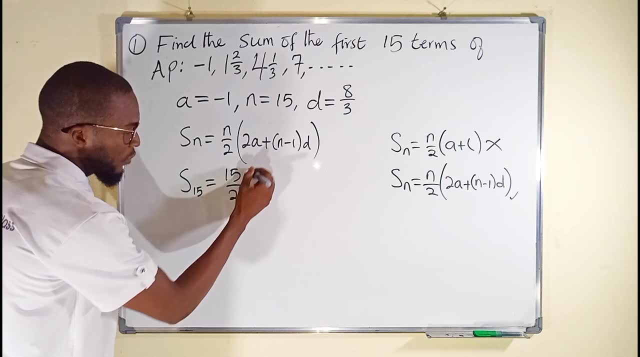 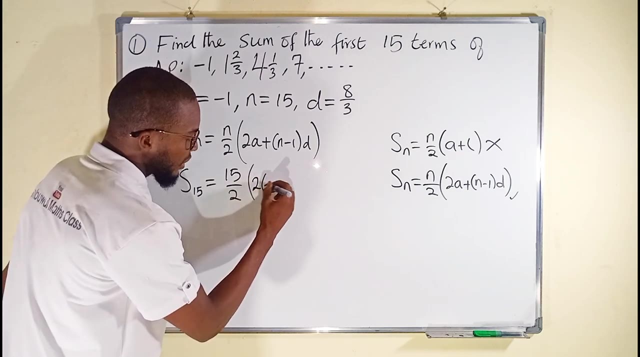 Let us substitute everything here: S 15 because N is 15.. Sum of the first 15 times equal to 15 divided by two. multiplied by two times A And A is negative one. So we have two Multiplied by negative one plus N is 15.. 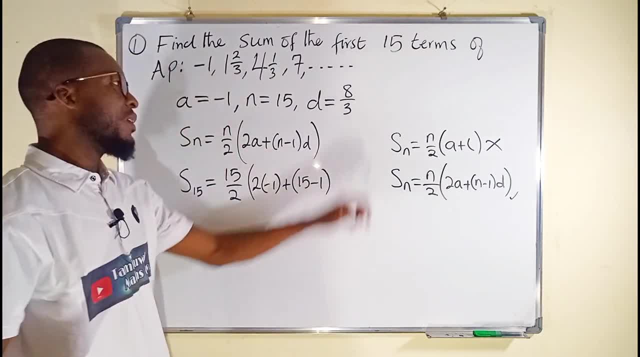 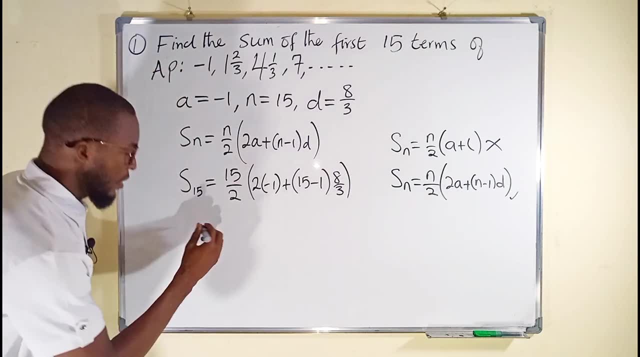 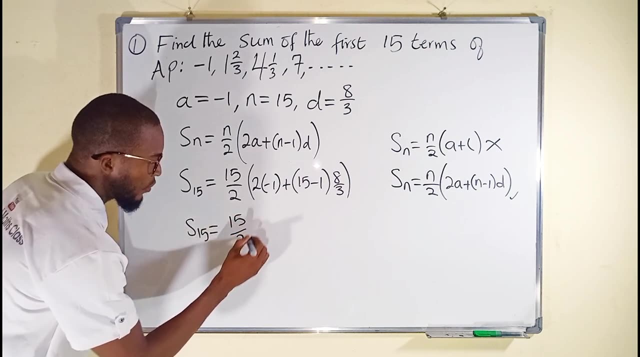 So we have 15 minus one. D is eight over three, So we have eight over three. S 15 would be equal to 15 divided by two. Here we have two multiplied by negative one. It is negative two. It is negative two. 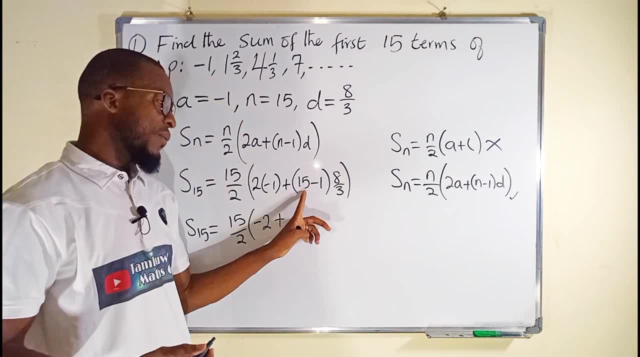 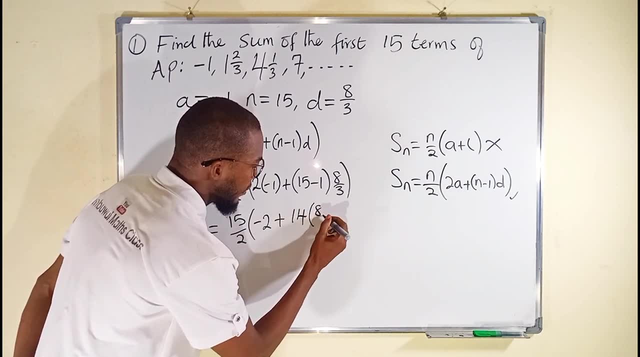 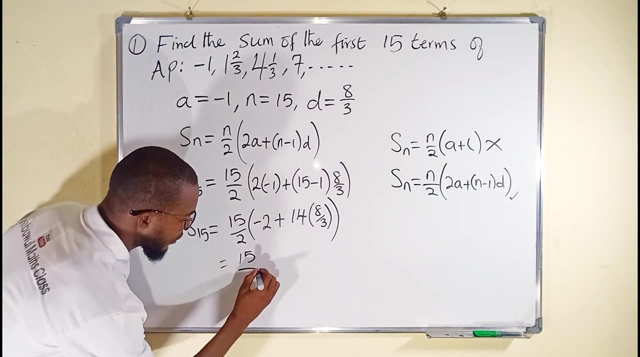 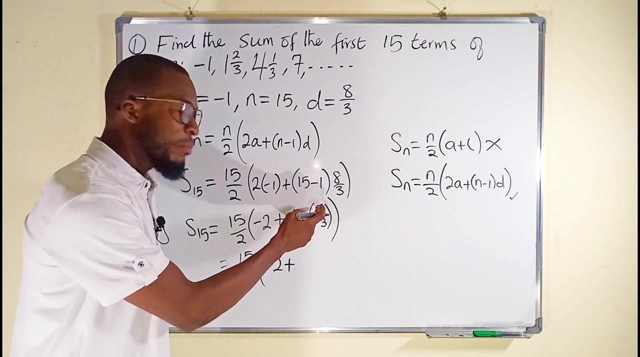 It is negative. two Plus 15 minus one is 14.. So we have 14 here. Multiplied by eight. over three, This is equal to 15 divided by two Multiplied by negative. two plus 14 multiplied by eight is 112.. 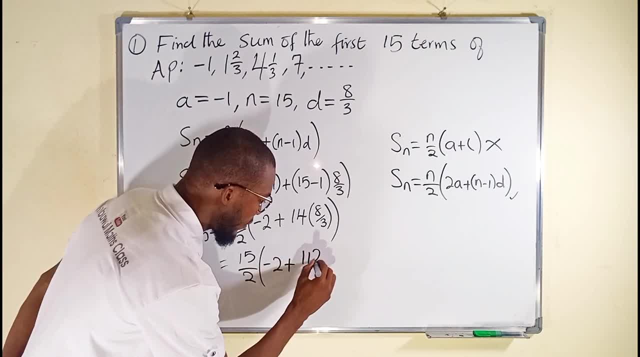 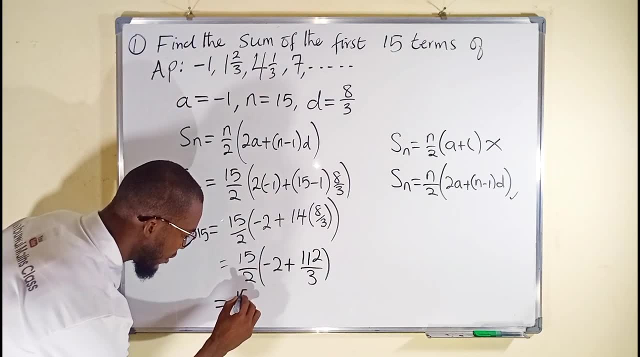 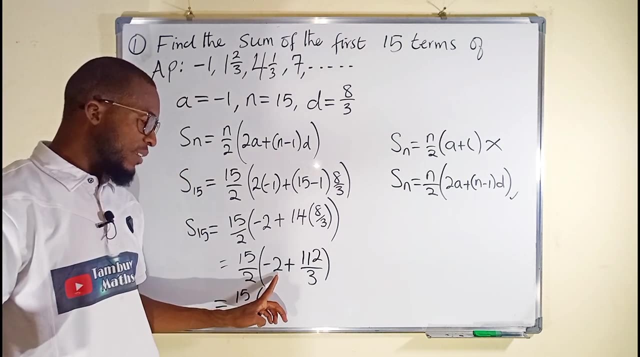 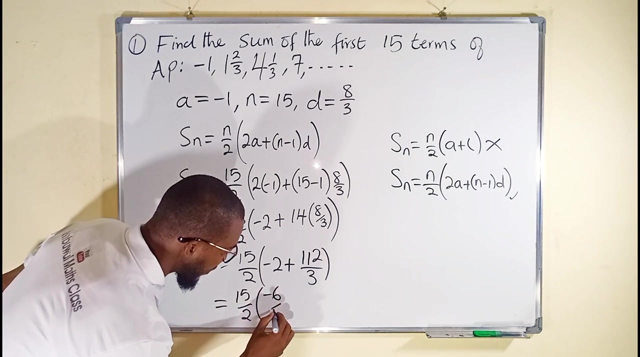 So we have 112.. Plus 112.. Divided by three- We are still simplifying- This is equal to 15 divided by two. Multiplied by, We can rationalize this as negative six over three. So this is negative six over three because we want to have a common denominator. 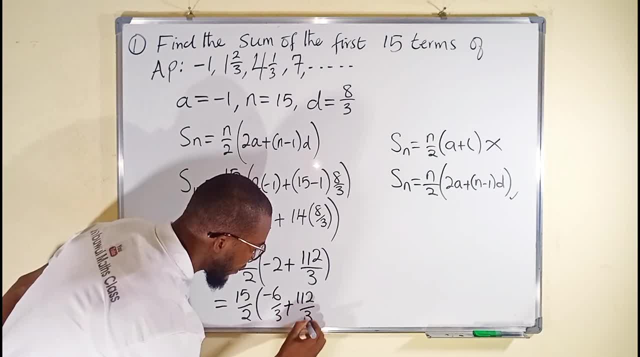 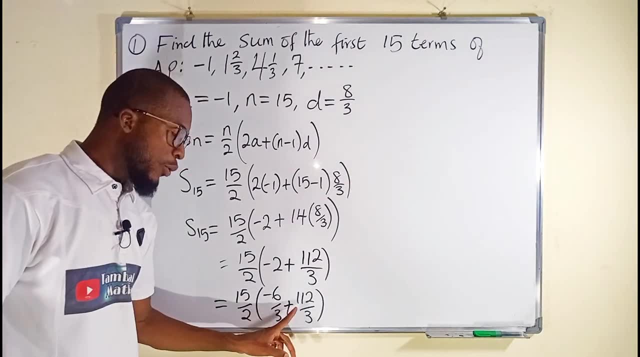 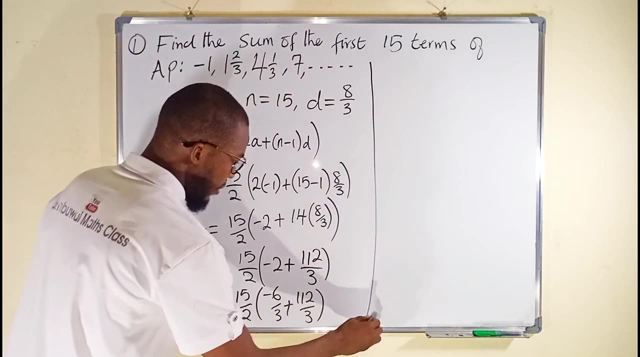 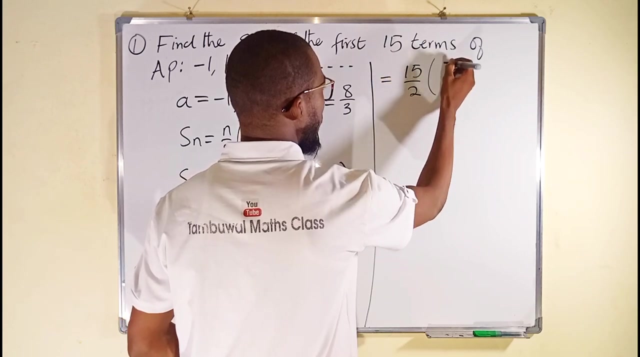 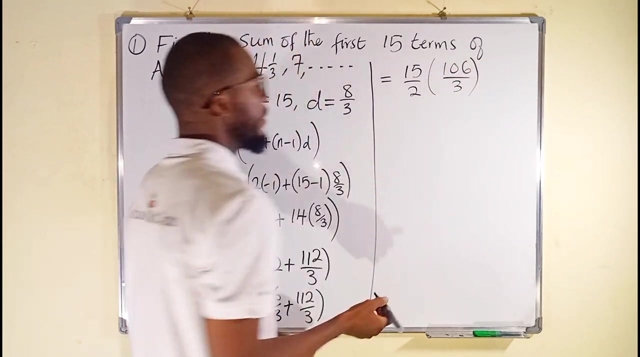 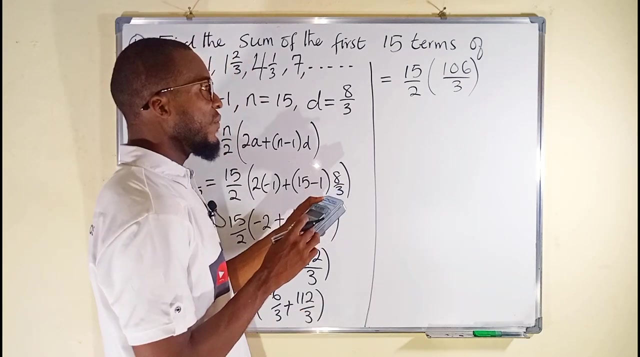 Plus 112, divided by three, Negative six plus 112 will give us 106.. So from here we have 15 divided by two multiplied by 106 divided by three. So now we are free to use calculator direct to multiply everything. 15 multiplied by 106 is 1590. 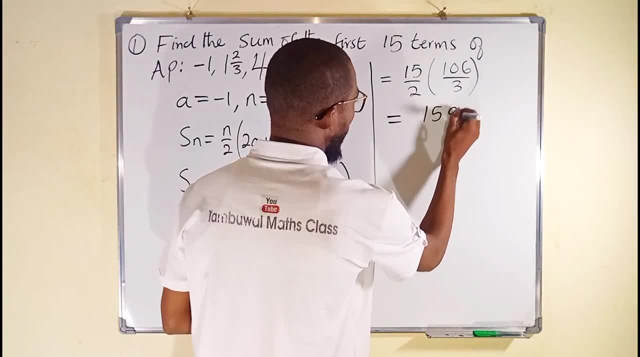 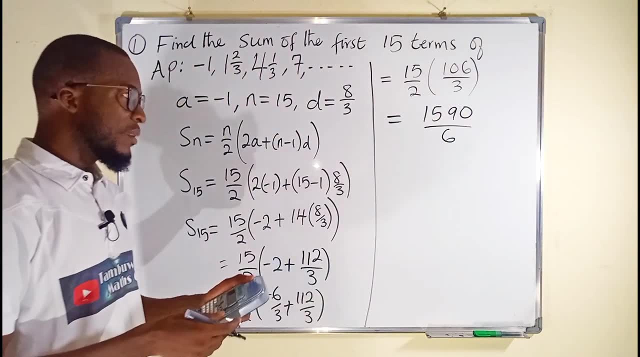 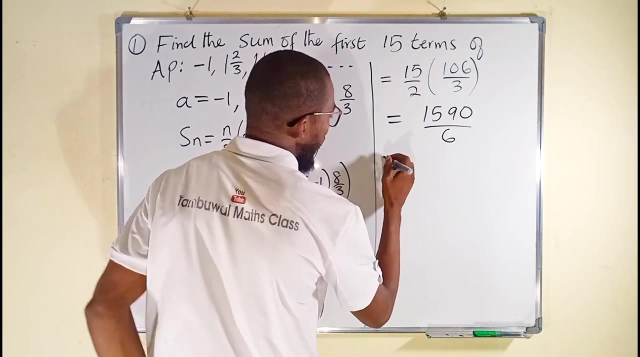 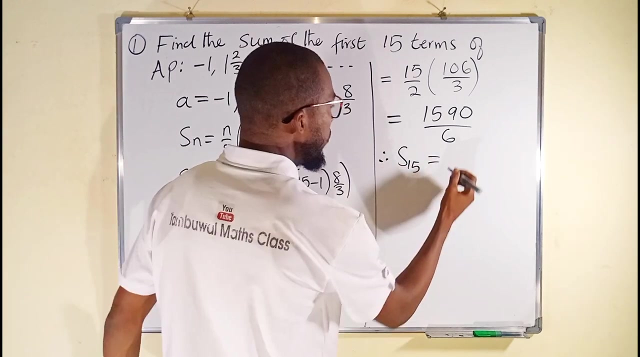 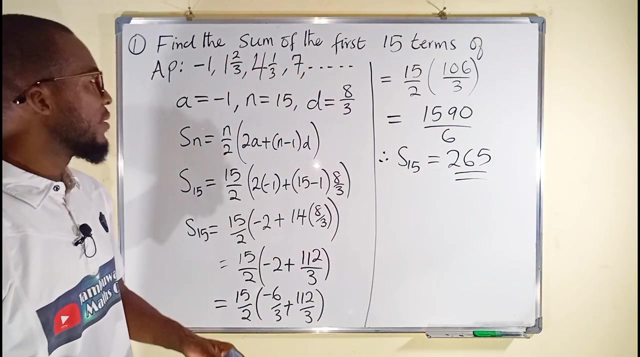 This is 1590.. And two multiplied by three is six. So we are going to divide that by six, Divided by six, And we have 265.. Therefore, S15 is equal to 265.. Therefore, the sum of the first 15 times in this sequence is said to be 265. 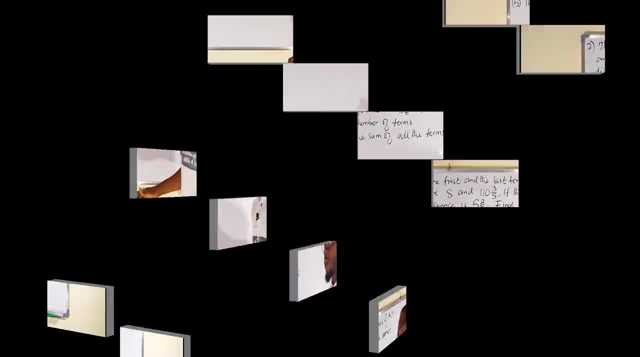 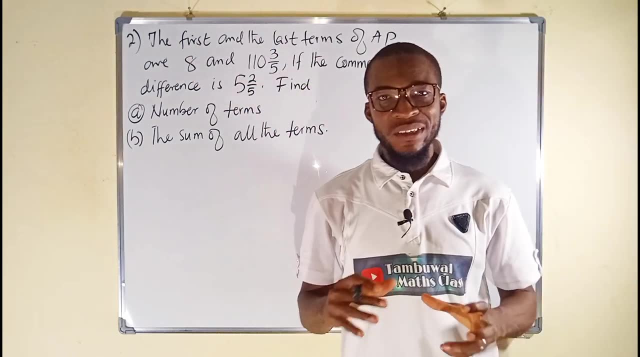 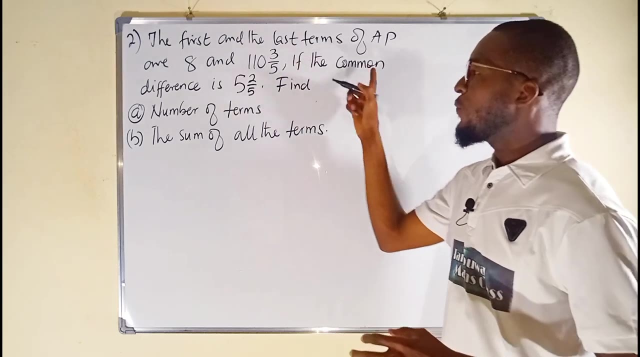 And this is the first question. Let us go to the second one. And here is our second question, Which says: The terms of an arithmetic progression sequence are given as 8 and 110, 3 over 5.. If the common difference is 5,, 2 over 5.. 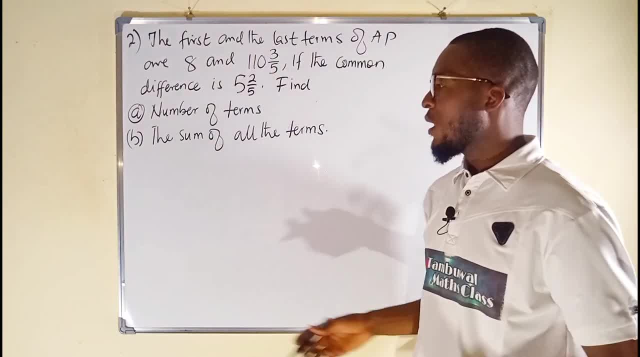 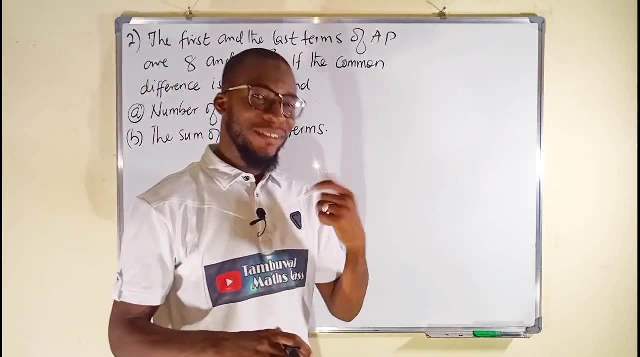 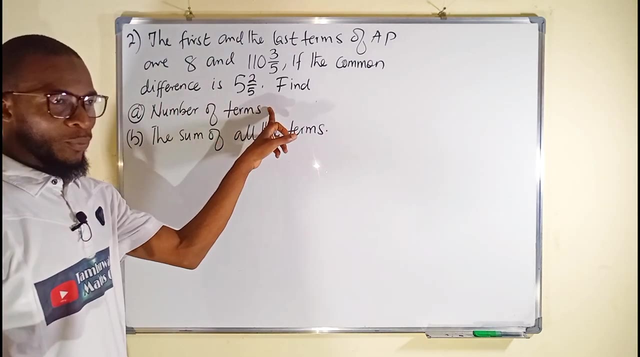 We are asked to find the number of times in this sequence And hence find sum of all the terms. All right, Remember that formula for finding the n terms of an arithmetic progression is very important here While solving the first problem here, And we can use that formula for sum of terms. 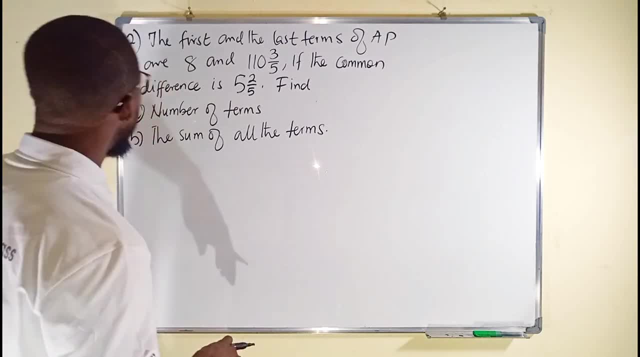 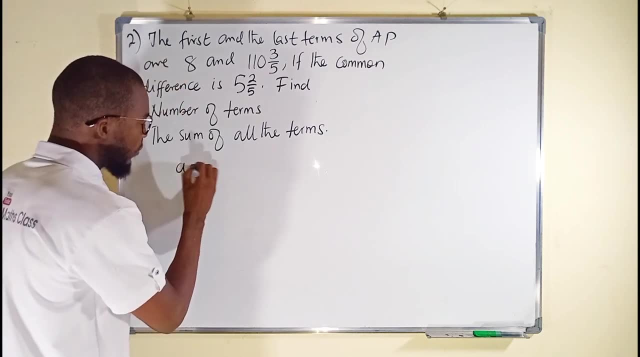 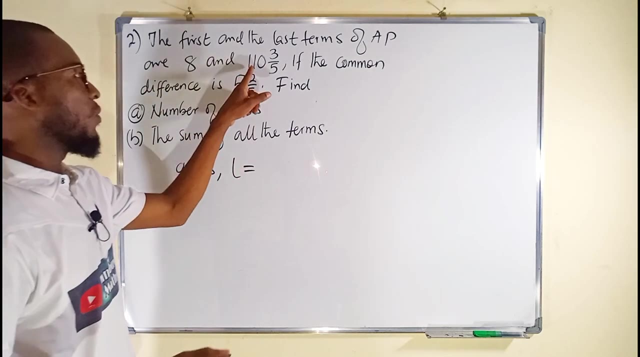 To find the solution to the second problem here. So let us first of all write our data. We are given First term E, Which is 8.. We are given the last term, L, Which is 110,, 3 over 5.. 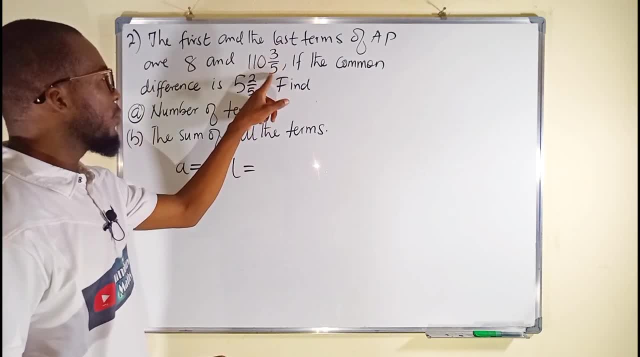 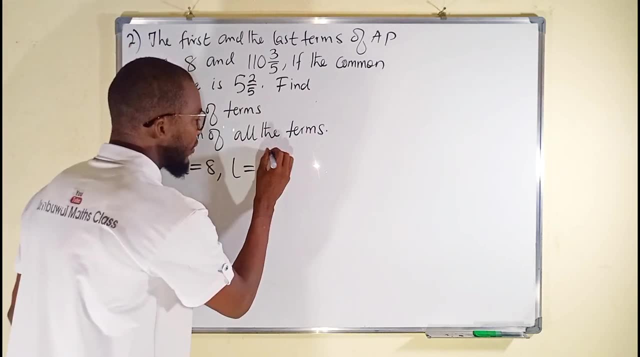 Which we can convert to improper fraction: 5 multiplied by 110 is going to be 55.. Plus 3 is 553.. So we have 553 here Divided by 5.. But other thing again, We are given the common difference. 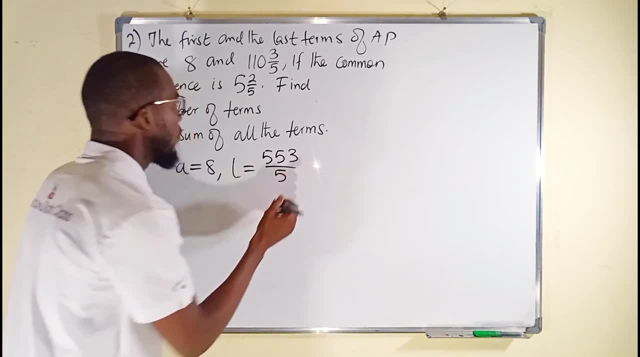 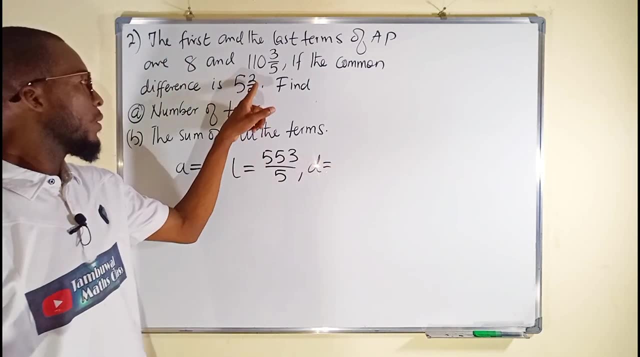 Which is D As 5.. 2 over 5.. 5 times 5 is 25.. Plus 2 is 27.. So we have 27. Over 5.. All right, Remember We are solving A. 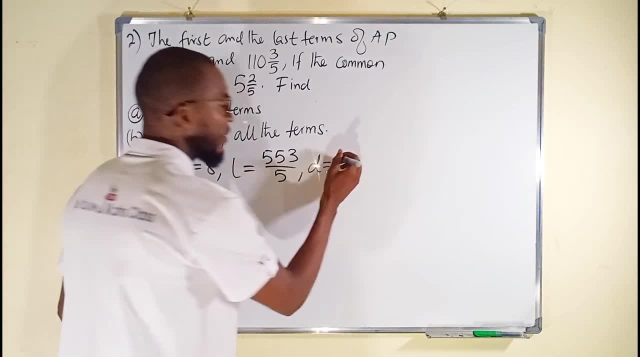 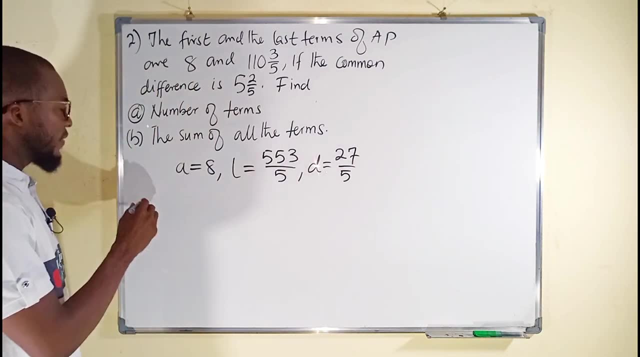 5 times 5. Plus 2 is 27.. So we have 27. Over 5.. All right, Remember We are solving A 5. 5. 5 times 5 is 27.. 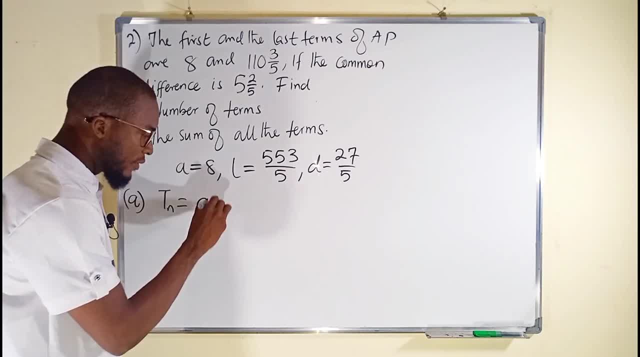 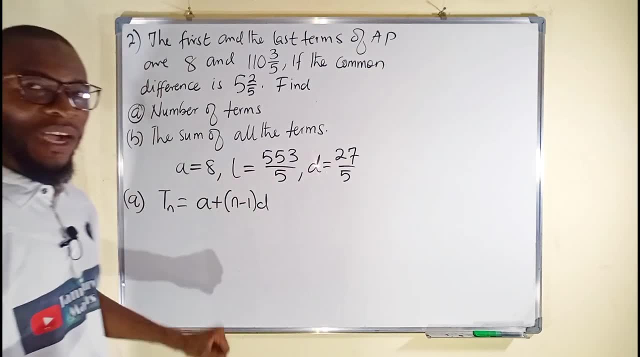 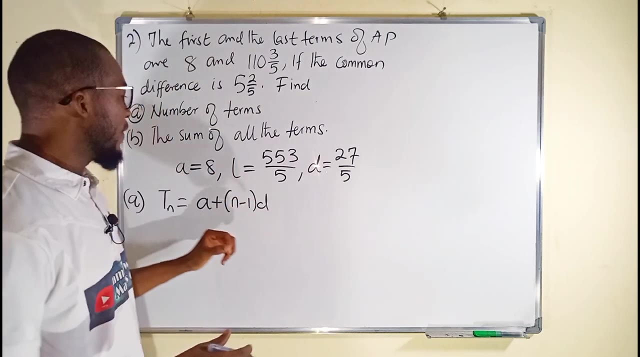 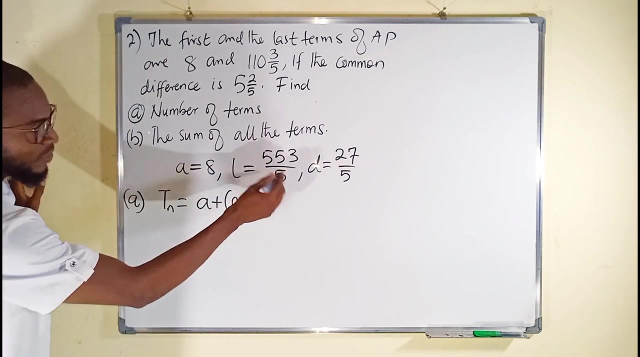 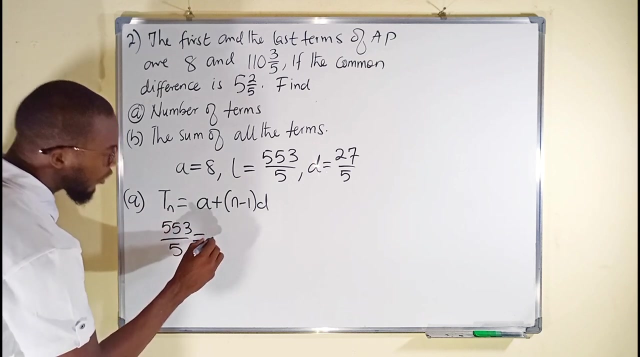 Plus 5 is 27.. So I Cer Makes 1.. So we are Example, So 0.. Since mean: Come To BR: 1.. 3 divided by 5.. This is equal to a, which is 8 here plus n, which we are looking for. 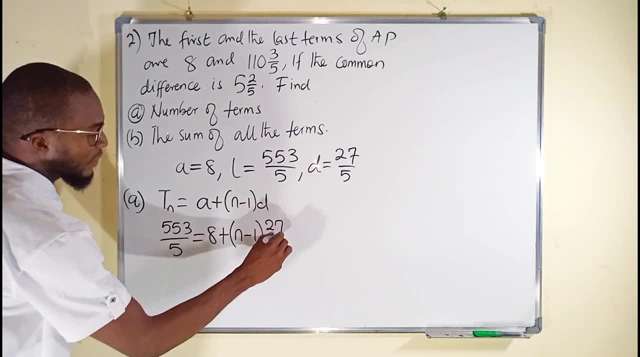 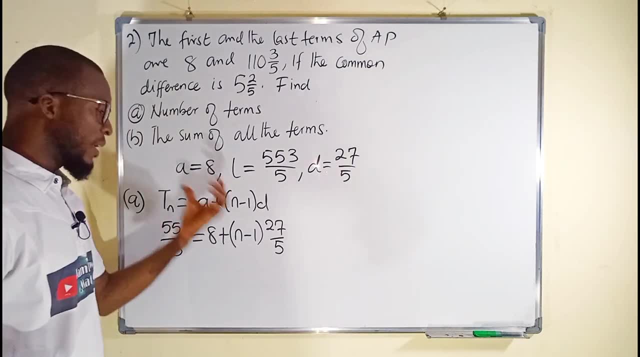 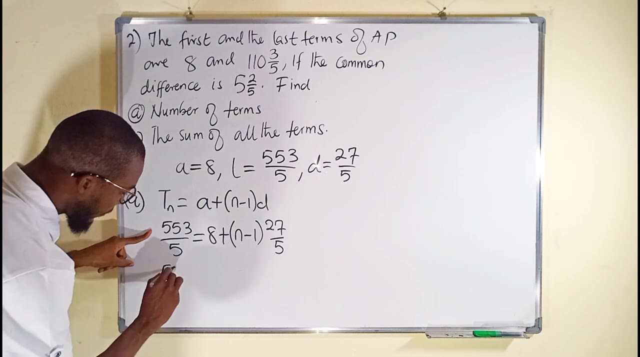 but d is 27 divided by 5.. Okay, first of all, let us clear the fraction by multiplying every term by 5.. If you multiply this by 5, 5 will take care of the 5, leaving 5 5 3. 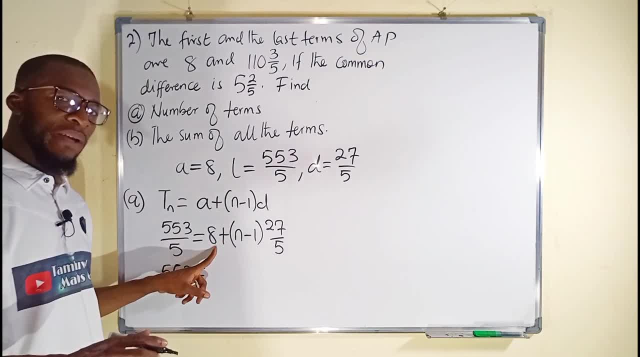 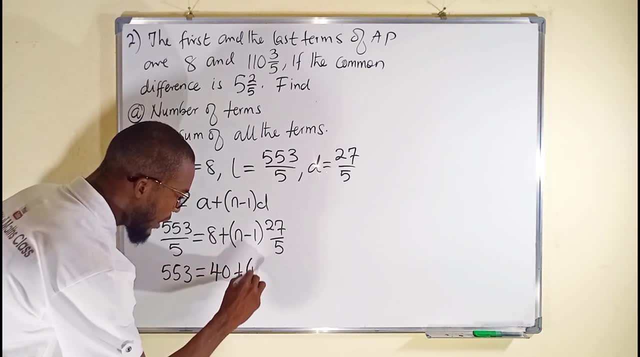 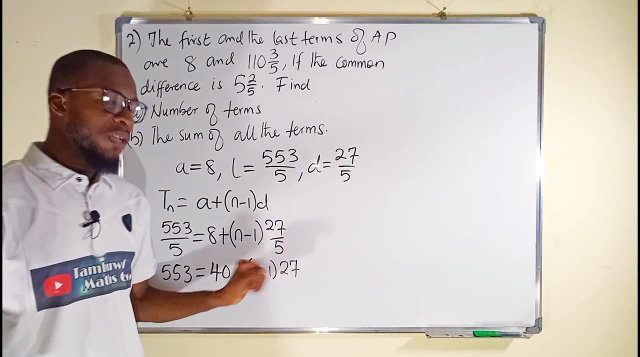 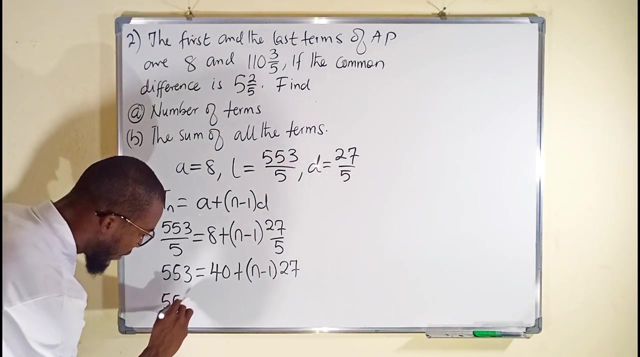 equals. if you multiply this by 5,, 8 times 5 is 40 plus n, minus 1 times 27, because 5 will cancel the 5.. So now let us take this 27 and distribute over. We have 5, 5, 3 equals 40 plus 27 n. 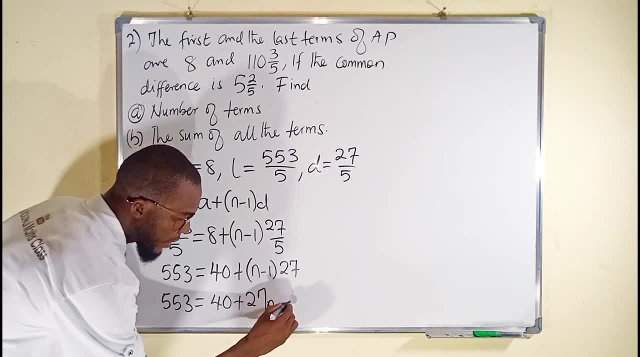 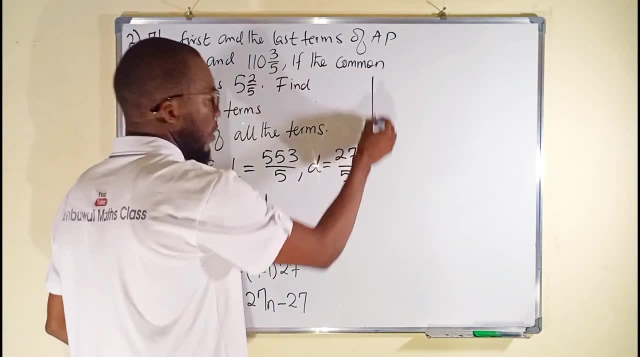 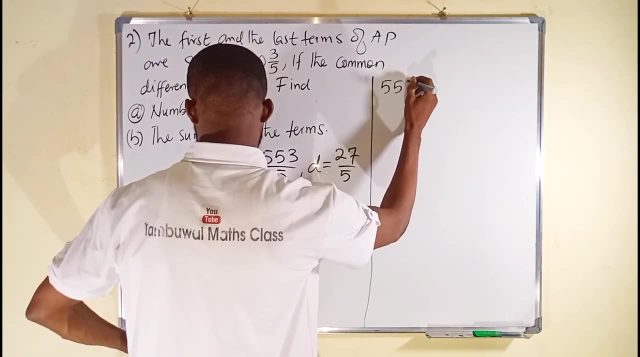 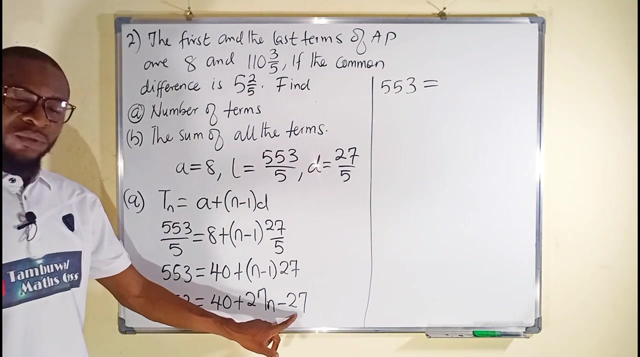 minus 27.. Let us collect the like times From the left hand side. we still have 5, 5, 3 and this is equal to: we have like times here. 40 minus 27 is going to give us 13.. So we have 13.. 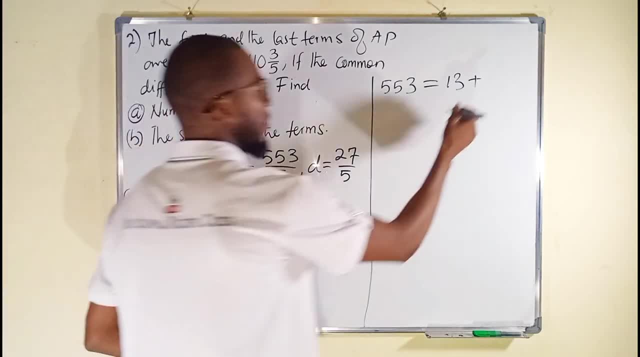 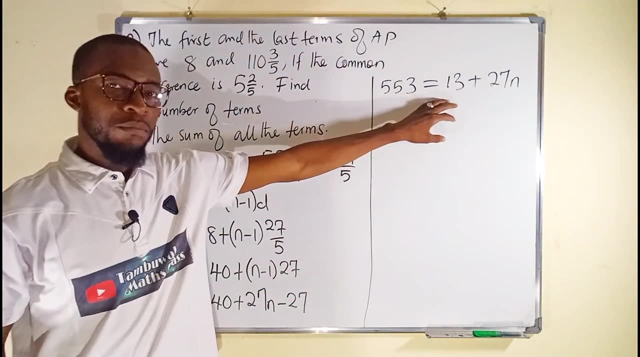 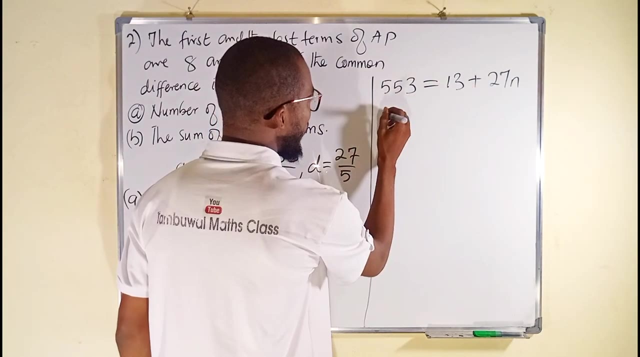 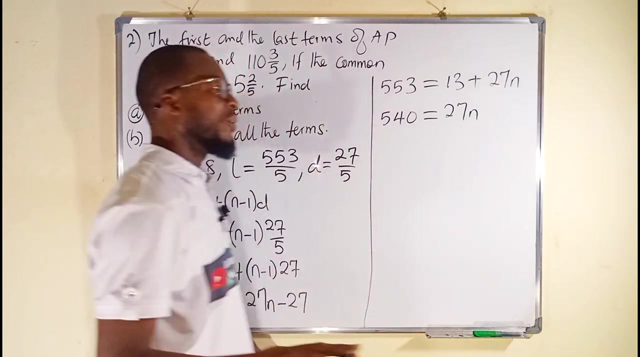 Plus 27 n, We have 27 n. Now we can bring our 13 backward, It becomes negative. We have 5, 5, 3 minus 13, which is going to give us 5- 40 and this is equal to 27 n. To find the number of times we 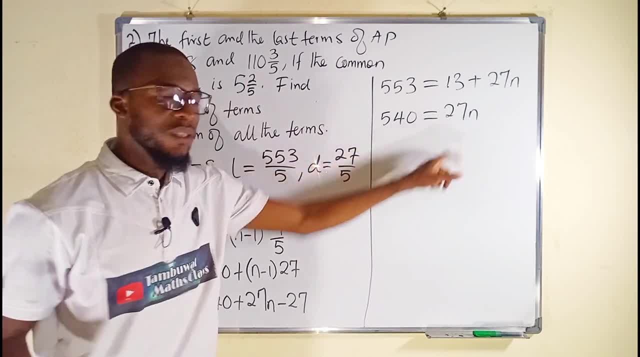 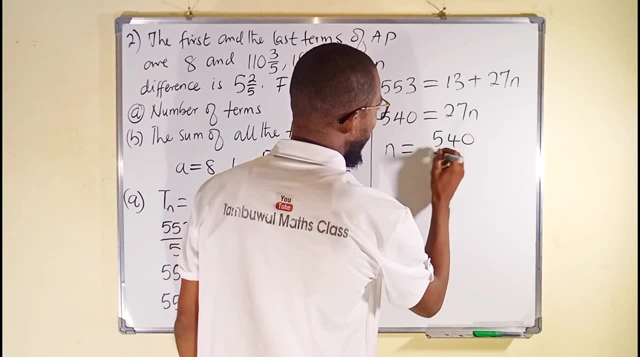 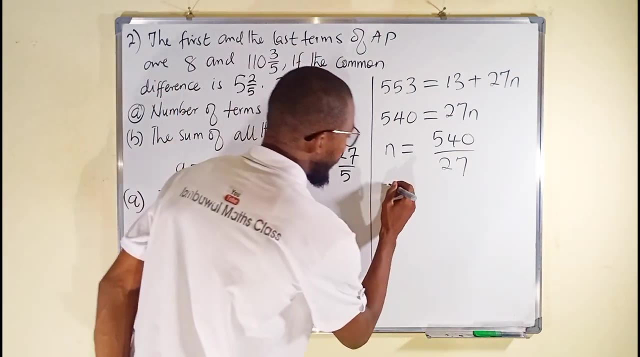 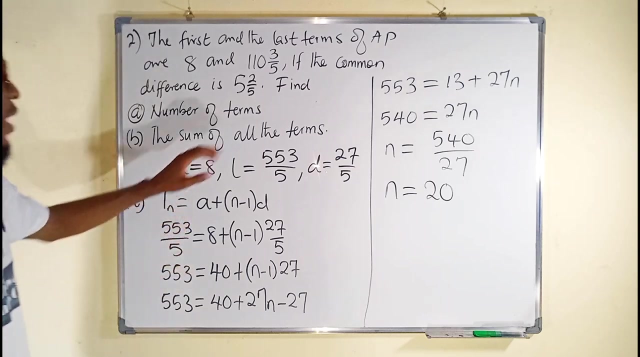 can now divide both sides by the coefficient of n, which is 27.. So n finally, which is our number of times, is 5: 40 divided by 27, and 5: 40 divided by 27 is equal to 20.. Therefore, the number of times in this sequence is said to be 20.. All right, we have just 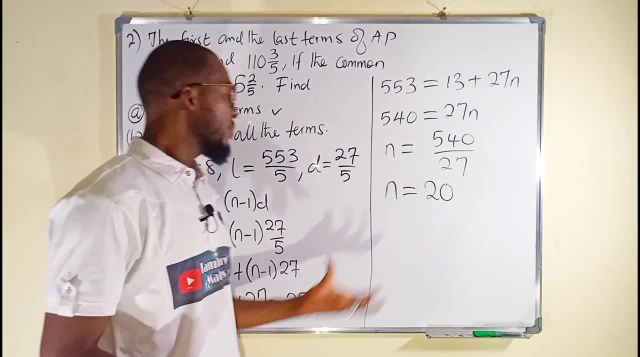 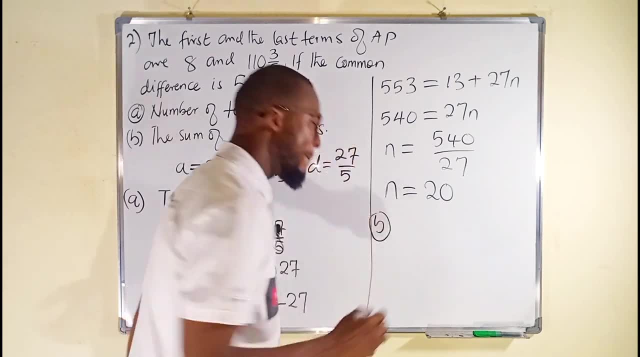 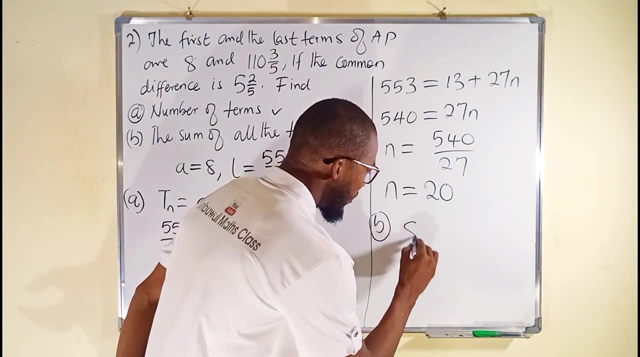 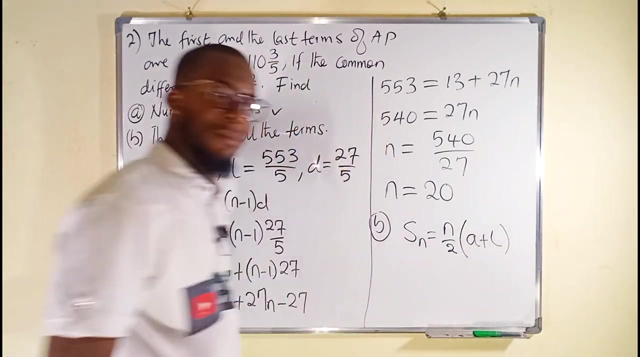 find a solution to this. solve question. Secondly, we want to find some of all the terms. Remember, if you are given the first and the last time, you can always use that formula that says, as n is equal to n over 2 multiplied by a plus n, Because we have obtained the number of times to 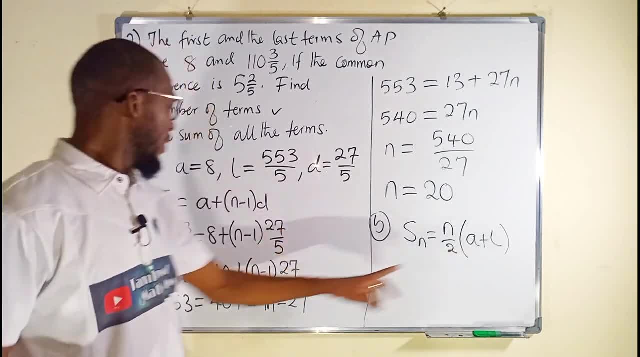 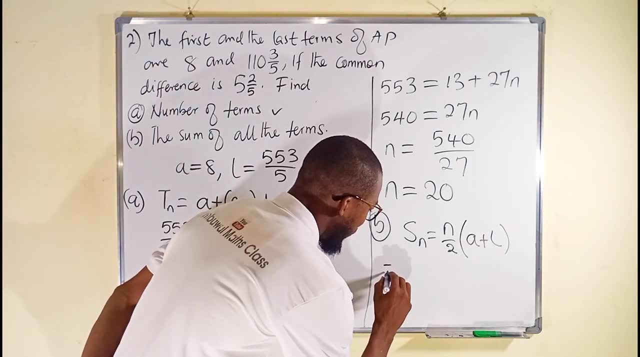 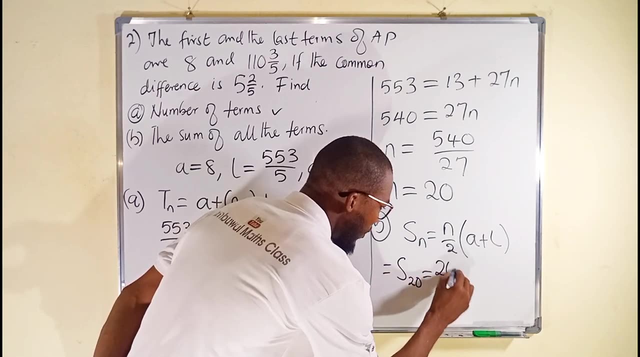 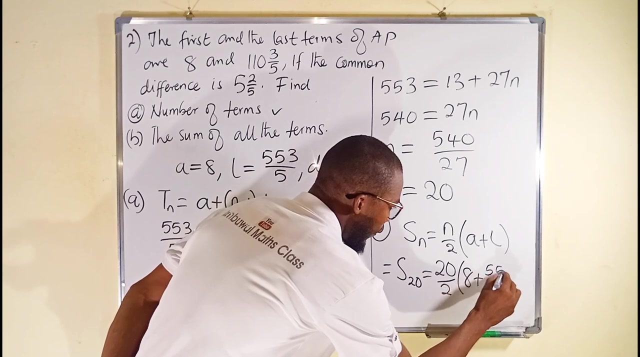 be 20. we can just plug it here, Substitute for a, which is 8, and l, which is 5 5 3 divided by 5.. Therefore, sum of this 20 times will be equal to n, which is 20 divided by 2, multiplied by 8, plus 5 5 3. 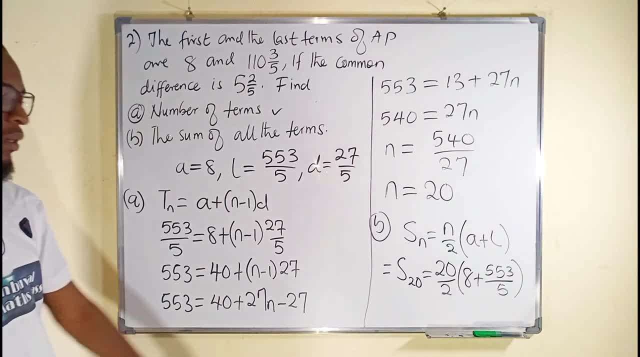 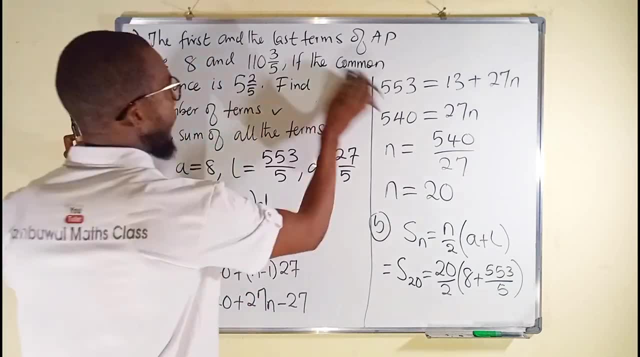 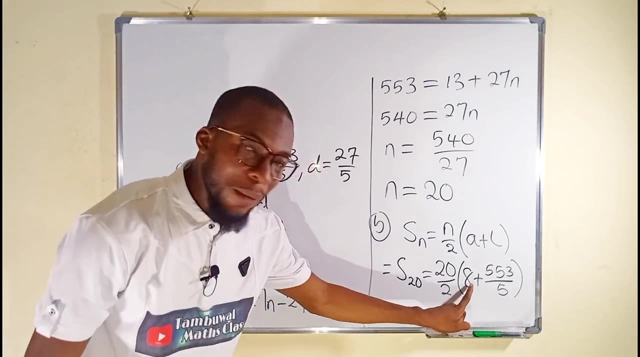 divided by 5.. This is what we need to simplify to obtain the sum of all the terms in this sequence, which are 20.. Okay, from here, Simplify the bracket. first, We can say 5 multiplied by 8, which is 40. Then, plus 5, 5, 3 is going to give us. 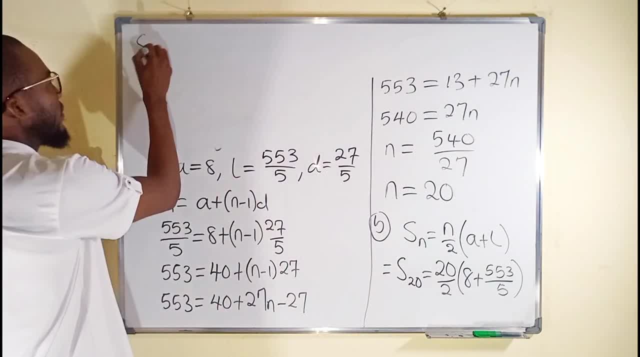 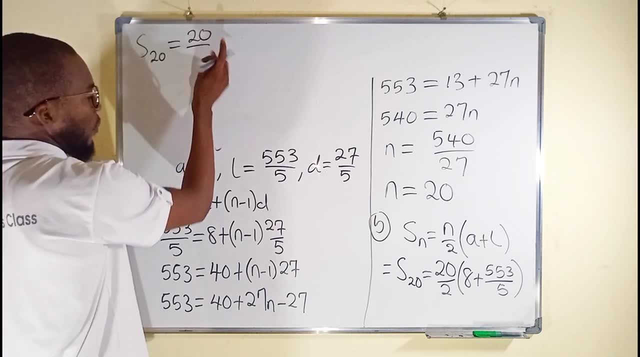 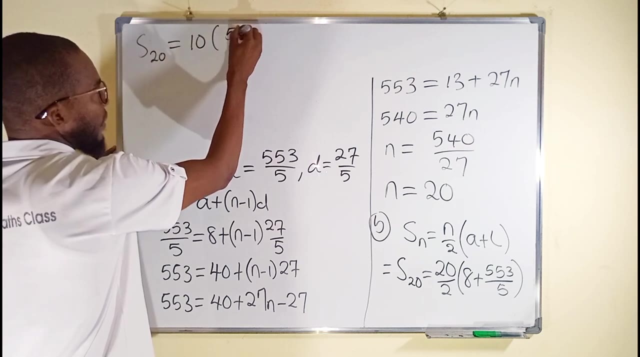 5, 9, 3.. So as 20, sum of the first, 20 times equal to 20 divided by 2, which is 10.. So this is 10.. Then multiply by 5, 9, 3 divided by 2..